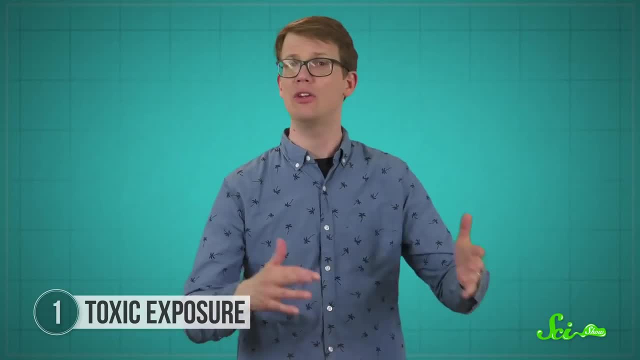 Wild birds have to be screened for lead poisoning each year and then treated if there's enough lead in their bloodstream, which requires a lot of time and energy. Scientists are hoping this won't have to go on forever, though, But it's not. 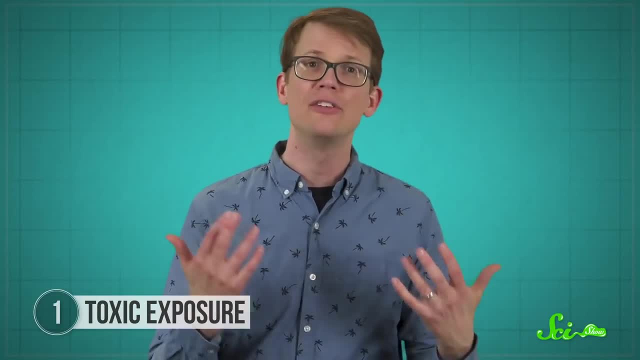 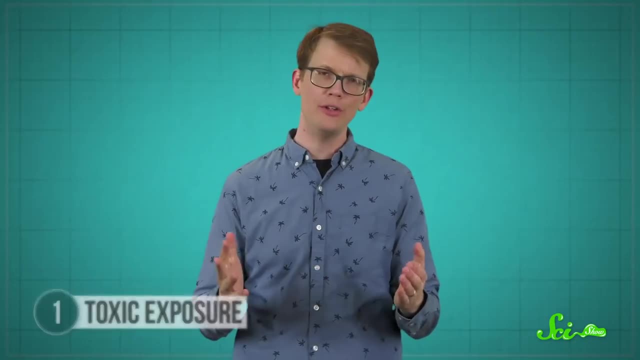 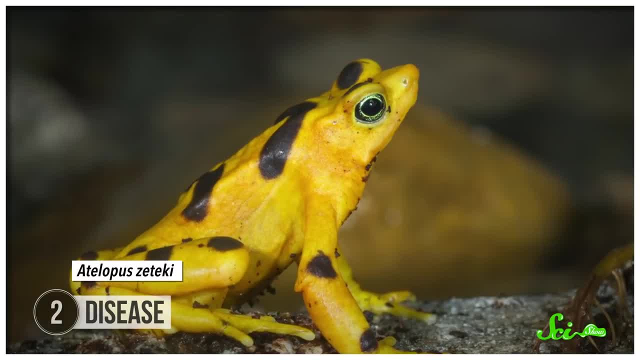 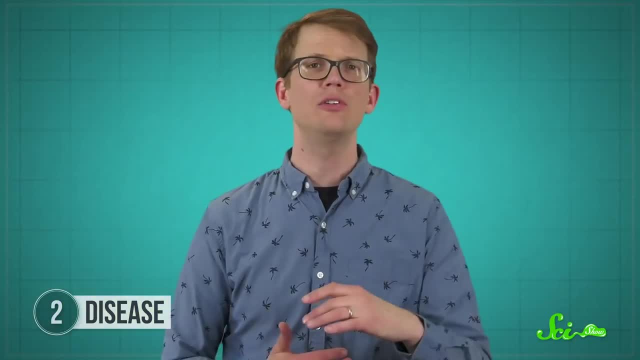 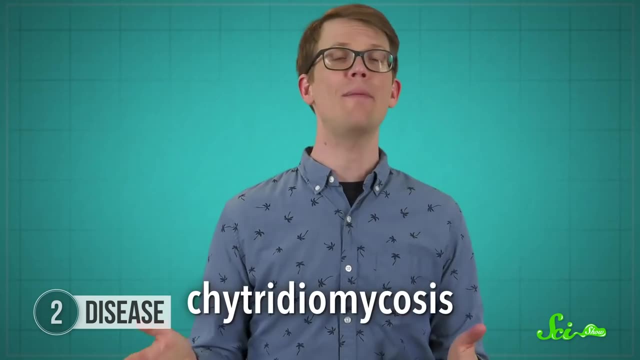 This frog is Panama's national animal And it packs a toxic punch so powerful that one individual contains enough toxin to kill 1,200 mice. It was once found near forest streams along the slopes of Panama, But the spread of the fungal disease chytridiomycosis has now wiped out the entire wild population. 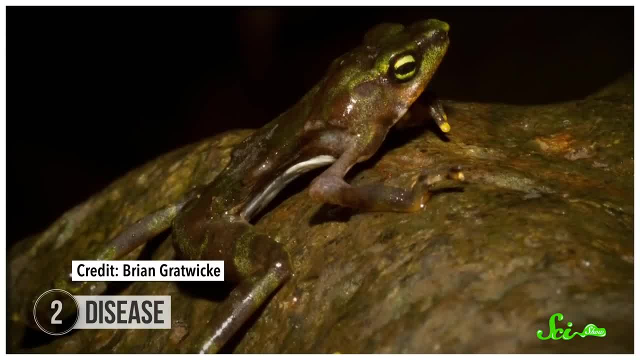 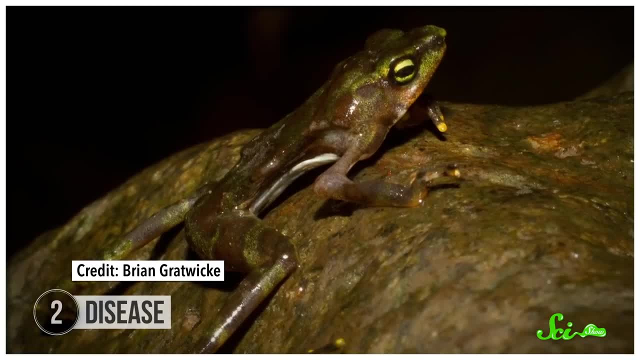 The chytrid fungus is a serious killer. It causes microscopic changes in amphibian skin so that it becomes really thick, And since amphibians absorb water and salts through their skin, they can't get rid of their skin and sometimes even breathe through it. this typically causes heart failure or 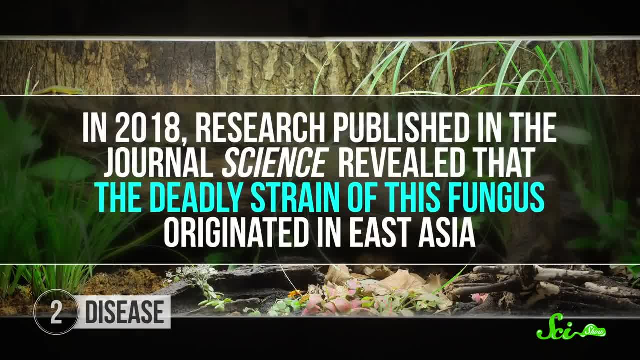 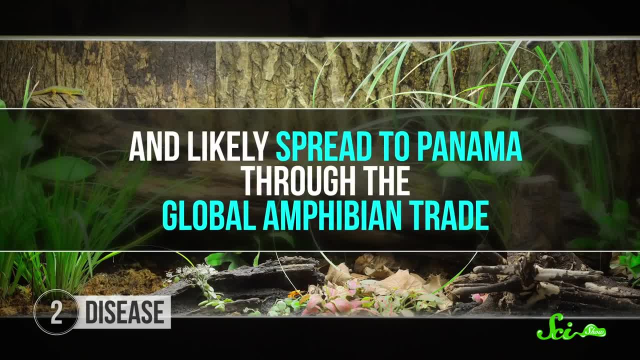 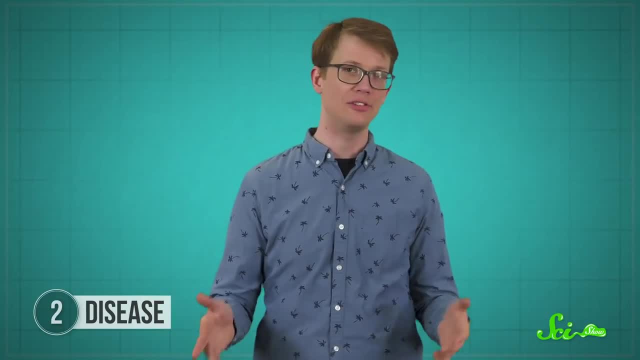 suffocation. In 2018, research published in the journal Science revealed that the deadly strain of this fungus originated in East Asia and likely spread to Panama through the global amphibian trade. So yeah, this one is probably our fault too. As far as we know, these frogs now only exist in managed breeding facilities and zoos. 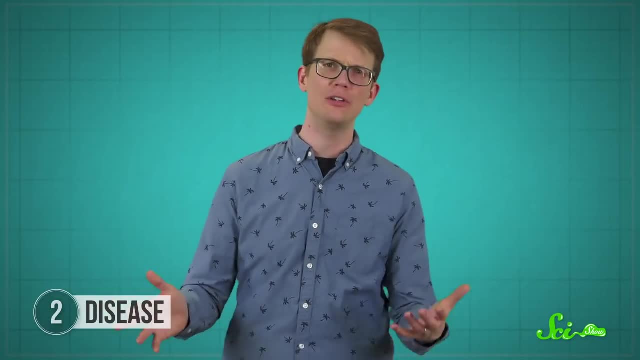 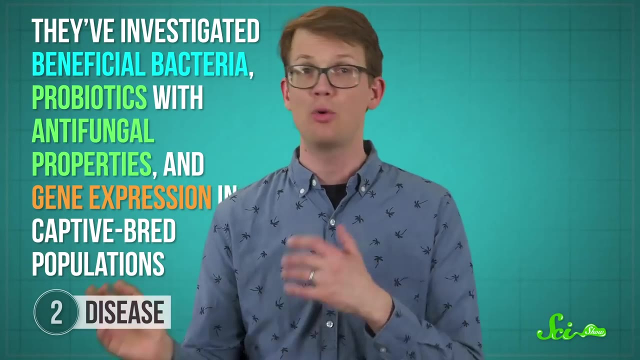 But researchers have been working on ways to protect future frogs if they're ever reintroduced to the wild. Their work is incredibly complex and they've investigated beneficial bacteria, probiotics with anti-fungal properties and gene expression in captive-bred populations. 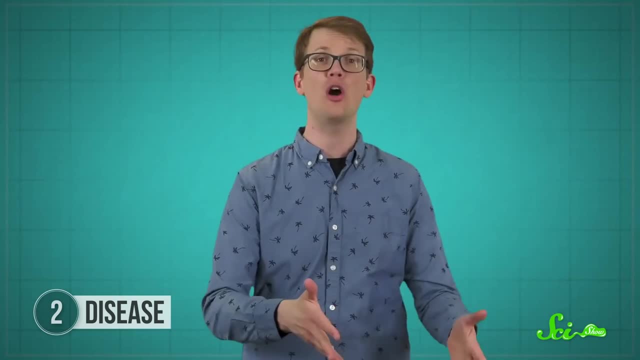 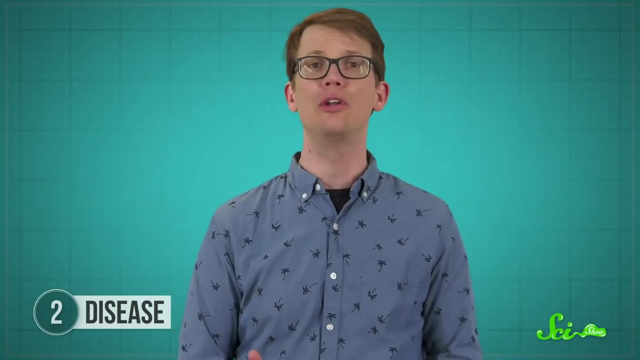 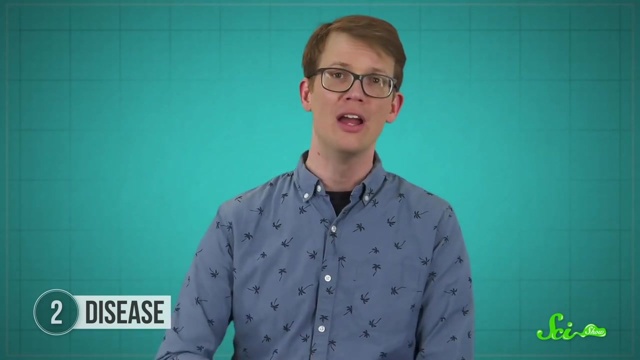 They're even perfecting techniques to extract and freeze frogs' sperm to hopefully add some genetic diversity to their gene pool. Although the future is very uncertain for the Panamanian golden frog, this research could greatly benefit other amphibian species too, because it's not just the golden frog. 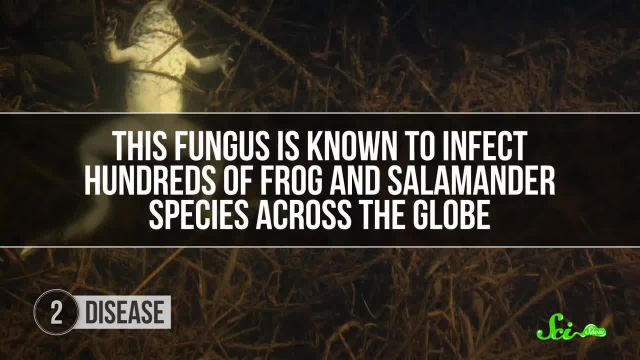 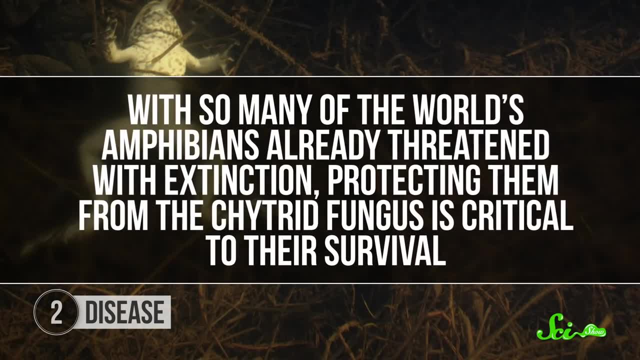 that's in such dire straits. This fungus is also known as the golden frog. This is known to infect hundreds of frog and salamander species across the globe And, with so many of the world's amphibians already threatened with extinction, protecting. 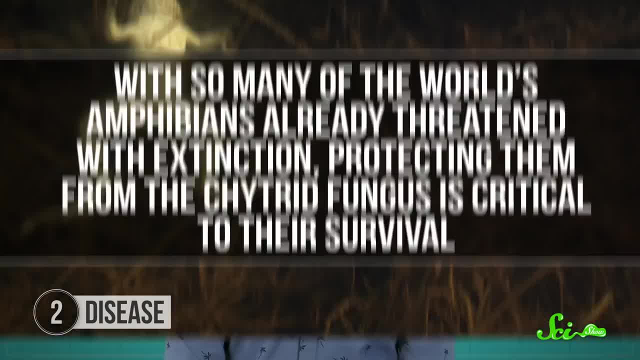 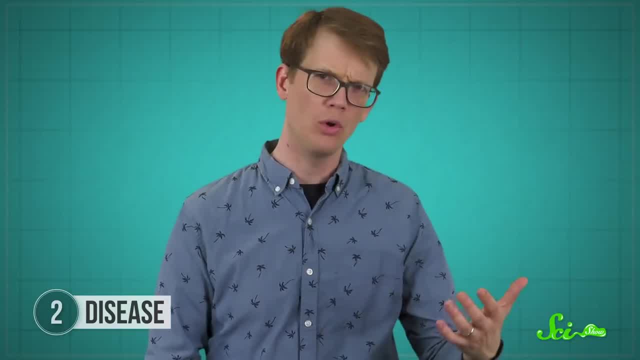 them from the chytrid fungus is critical to their survival. Many of these species are supported by a group called the Amphibian Arc, which supports amphibian care efforts around the world, But ultimately that's a lot of species to take care of. 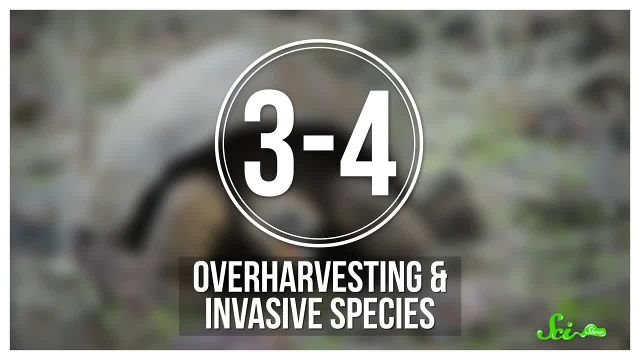 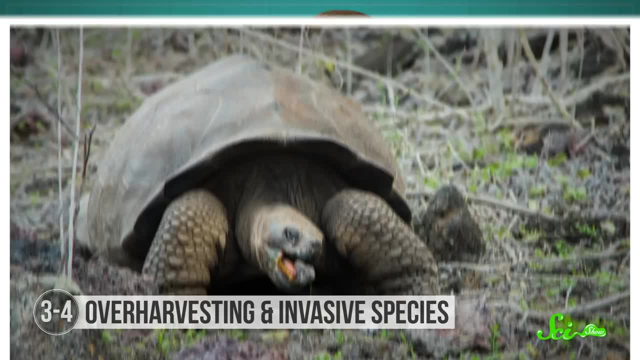 So the sooner we get them back to the wild the better. Sometimes, multiple factors are at play. Some species decline and their conservation reliance hinges on more than one threat. This is the case with one of the world's most famous shelled animals, the Galapagos. 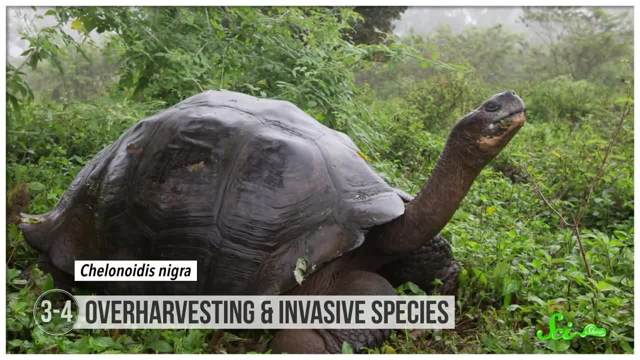 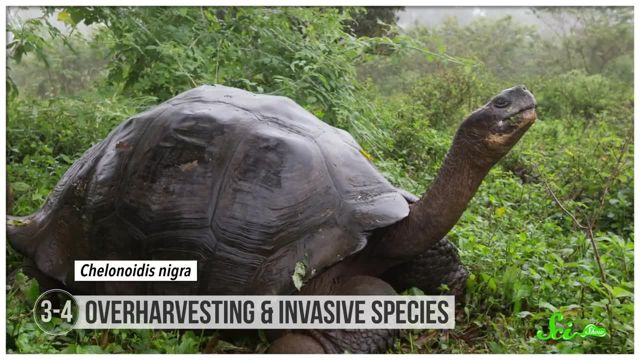 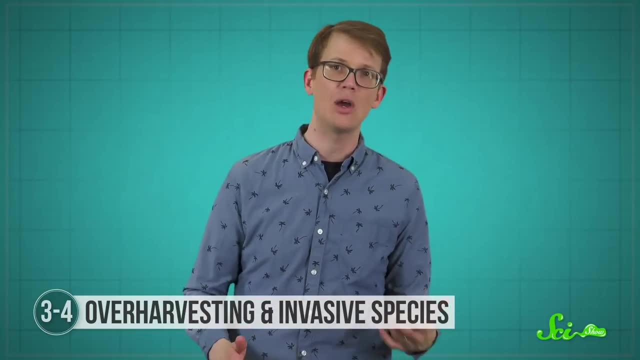 tortoises First. these gentle giants were dramatically over-harvested in the 1700s and 1800s, mostly for food or oil. So at least one species was already extinct before conservation efforts were even considered. Then, even after we stopped eating the tortoises, the threats didn't go away, because they 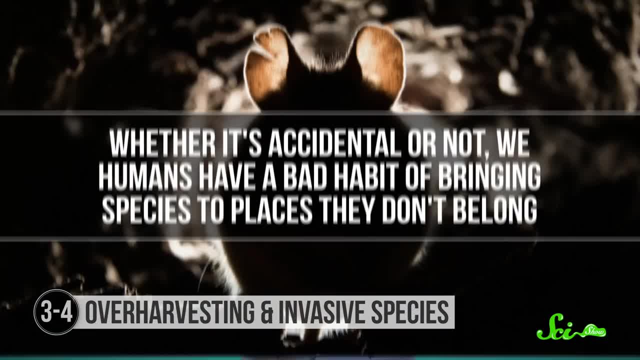 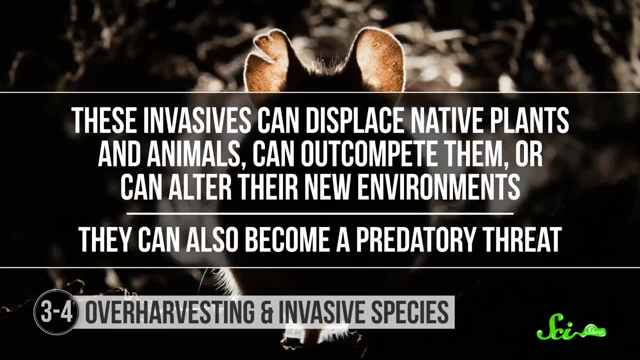 still had to deal with us With a bunch of invasive species. Whether it's accidental or not, we humans have a bad habit of bringing species to places that they don't belong. These invasives can displace native plants, and animals can out-compete them, or can. 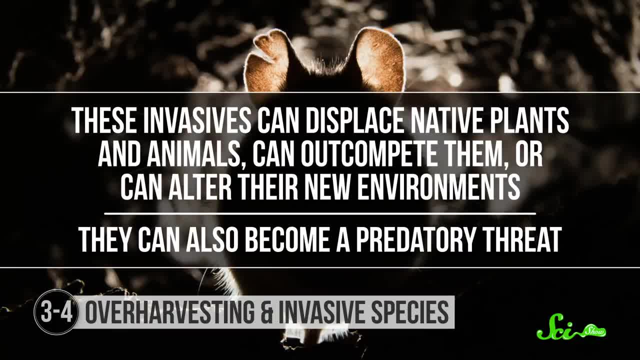 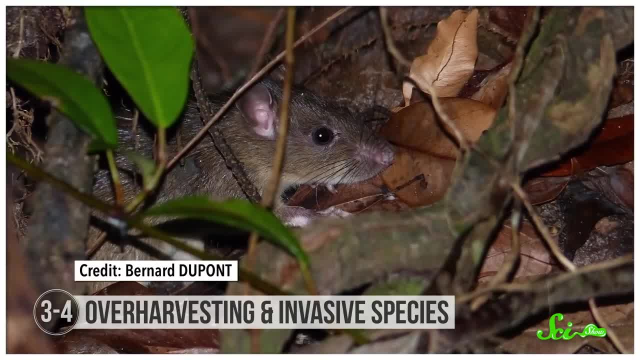 alter their new environments, They can also become a predatory threat, Or, in the case of the poor Galapagos tortoises, all of these things can be true. For example, black rats were introduced to the Galapagos Islands in the late 1800s, and 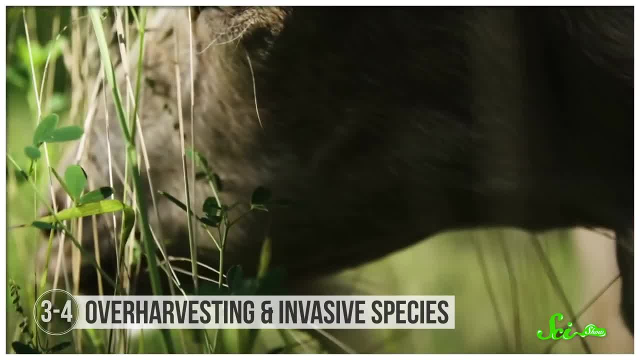 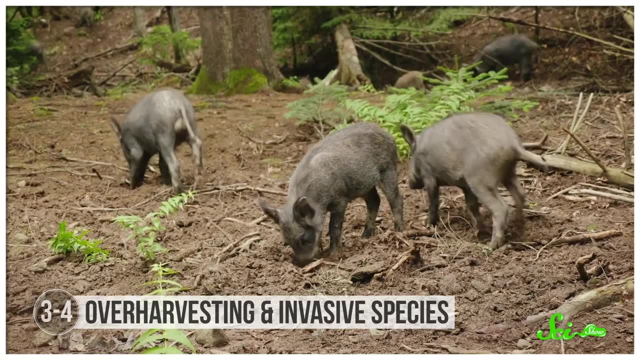 they've been eating tortoise eggs and babies ever since, And they've been eating tortoise eggs and babies ever since. Then goats were brought there and dramatically changed the vegetation that the tortoises depend on. Eventually, pigs were introduced and they started feeding on nestlings and eggs and 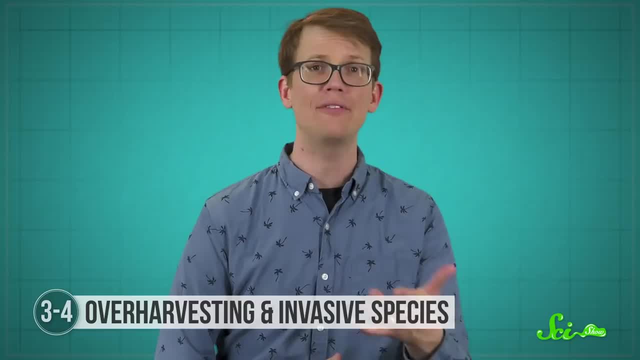 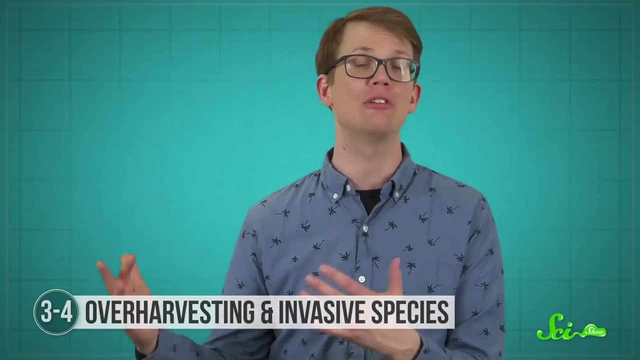 the list kept growing. Today, the tortoises also have to deal with an invasive ant that attacks hatchlings, and even invasive blackberries that prevent them from reaching food and breeding sites. I am sorry that we messed up your island so bad tortoises. 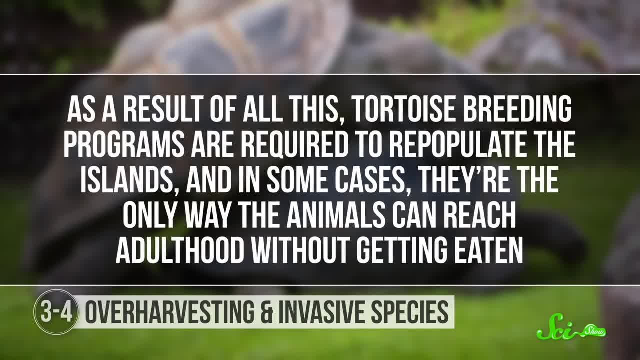 As a result of all this, tortoise breeding programs are required to repel the tortoises, And that's why we're here today. We're here to help you. We're here to help you. We're here to help you. 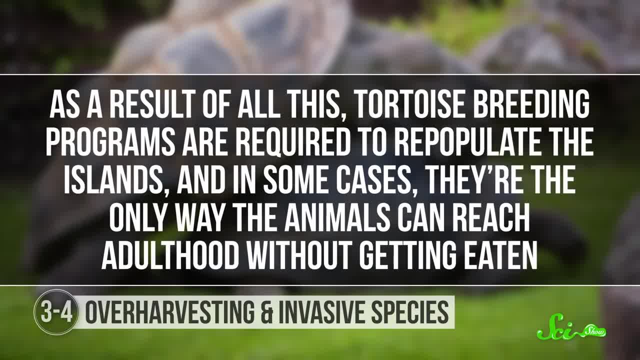 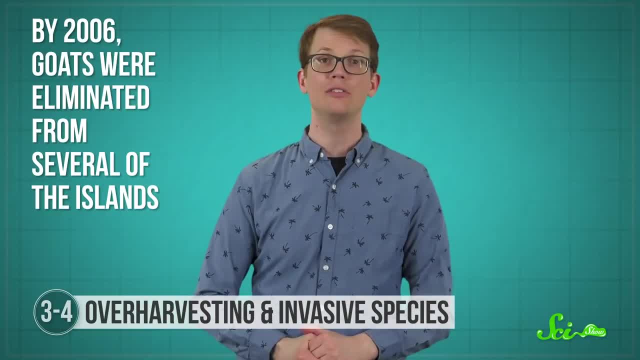 So far, these programs have been successful, But even better, we've also been able to deal with some of those invasives. By 2006,, goats were eliminated from several of the islands and black rats were eradicated from Pinzón Island in 2012.. 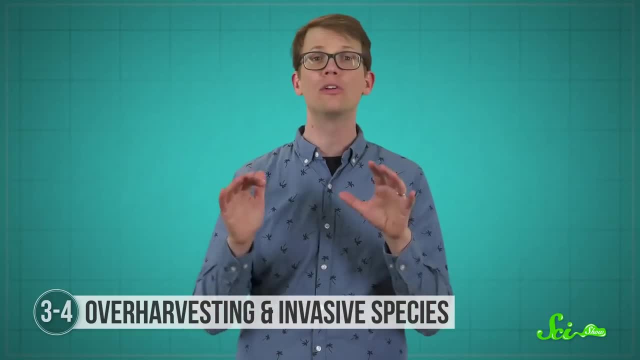 Then, two years later, wild-bred tortoise hatchlings were seen on the island for the first time in a century. All of these events have been an opportunity for the island to repopulate its own animals. That said, eradicating invasive predators from all of the islands was the only way that. 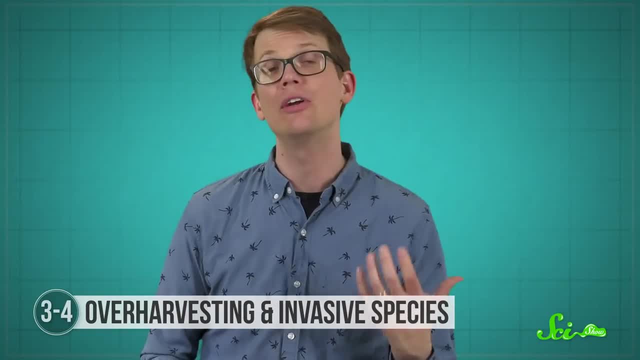 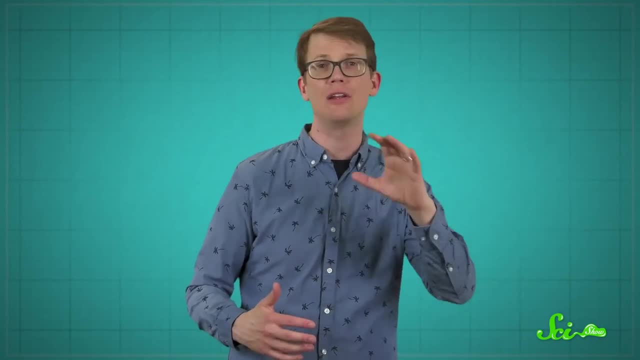 These islands may not be possible, especially for the larger islands, but there's still a lot of hope For the most part. we don't want other species to become reliant on us. We want them to survive and thrive all by their bad selves. 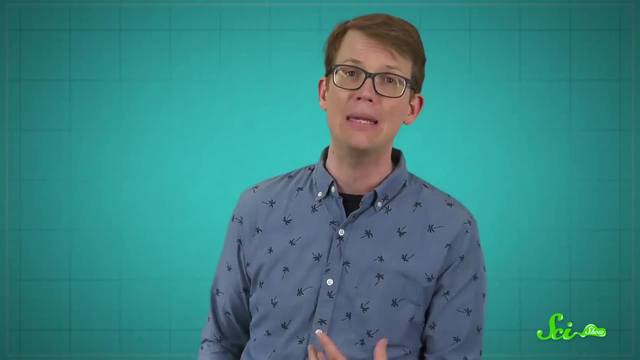 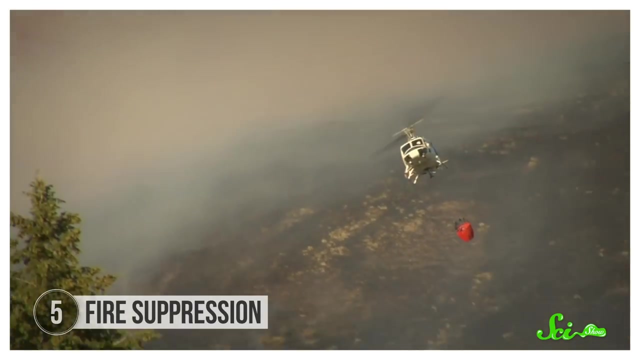 But sometimes the needs of a species don't overlap with what people want, And while it's a hotly debated topic, fire suppression is a key example of that. Fires are a normal part of nature and certain ecosystems rely on them to control forest. growth. The problem is those forests are often close to areas where people live, so they get suppressed or otherwise prevented, And the species that rely on those fires suffer. like the Karner blue butterfly, It was once found abundantly across 12 US states and one Canadian province. 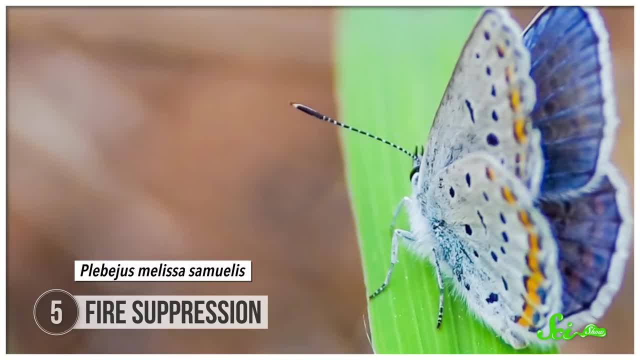 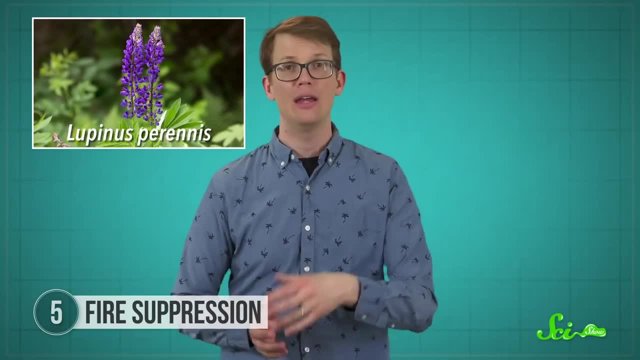 But in the last 15 years or so the population has dropped by 99%. That's because Karner blue caterpillars only feed on one type of plant- the wild lupine, And to thrive- the lupine nests- It needs fire. 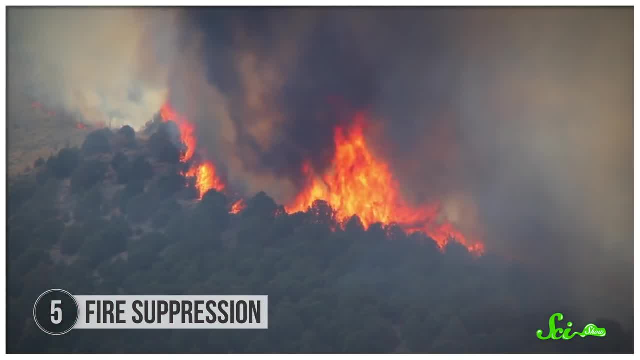 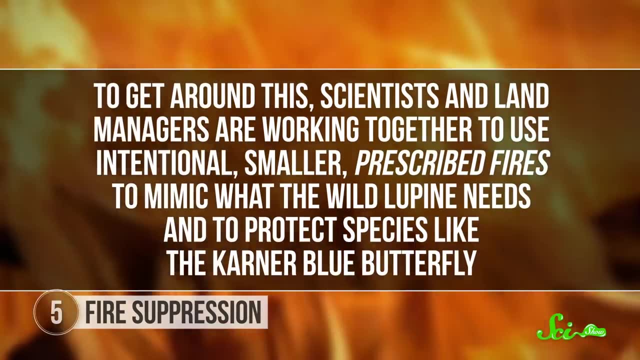 More specifically, it needs fires to open up forest canopies and allow sunlight to reach the ground. Otherwise it would be outcompeted by pines, oaks and shrubby vegetation. To get around this, scientists and land managers are working together to use intentional smaller, 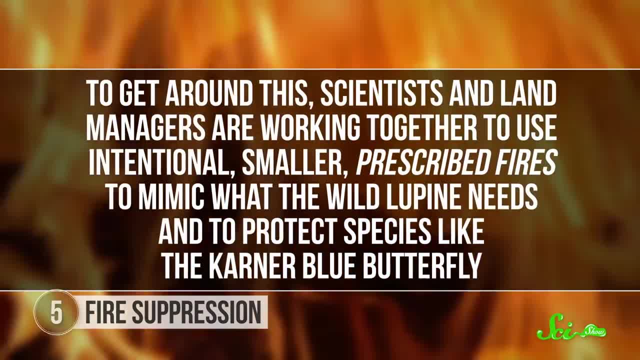 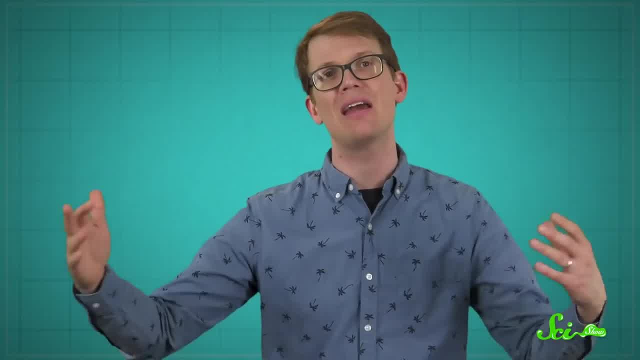 prescribed fires to mimic what the wild lupine needs and to protect species like the Karner blue butterfly. Like other conservation methods, it's something that takes a lot of time and effort, But many people argue this is the problem. This is the best option. 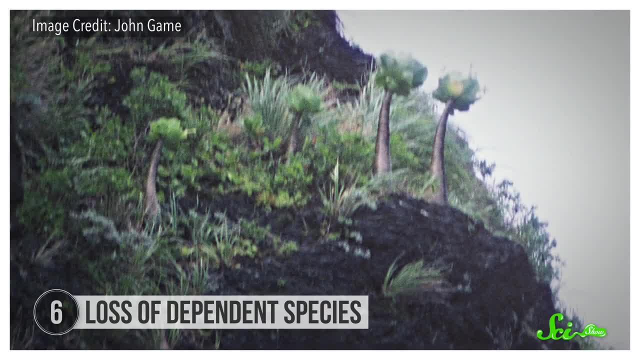 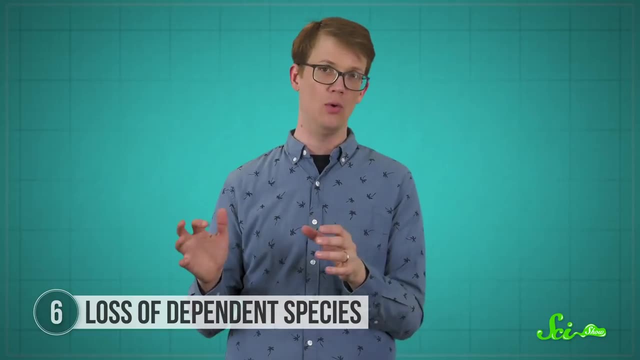 Finally, sometimes the loss of one species means the demise of another. This was true for a cliff-dwelling plant species commonly known as olula, Although it's also called cabbage on a stick, cuz look at it. This plant is endemic only to the Hawaiian islands of Kauai and Niihau. 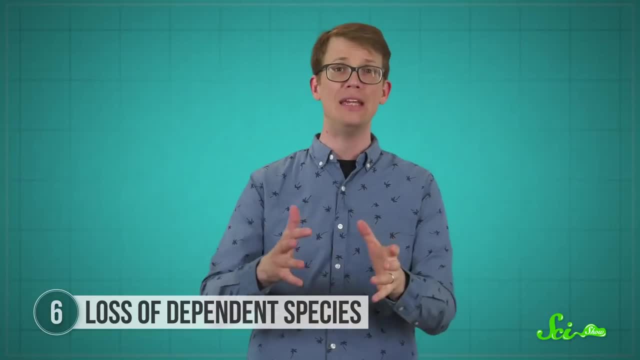 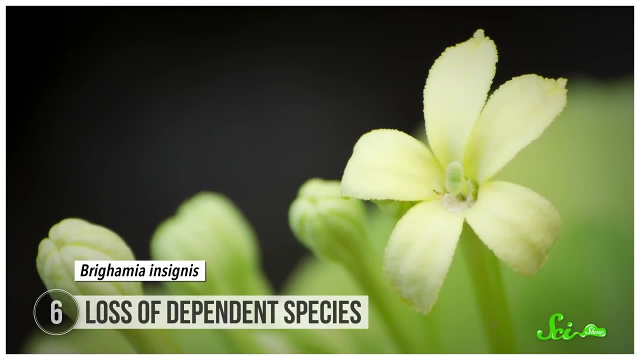 And unfortunately, its pollinator likely disappeared before we even knew for sure what it was. Based on the plant's flower shape, color and size, we now think it was likely a common plant species, But we don't know for sure. We don't know for sure. 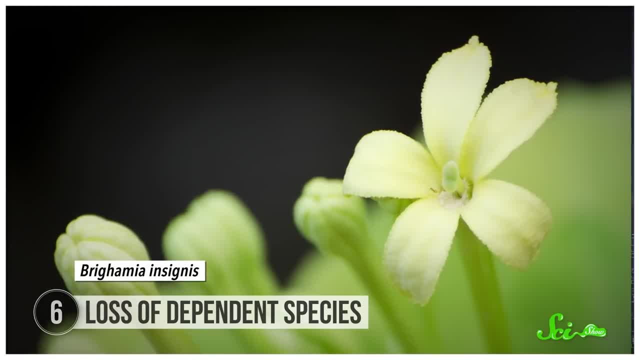 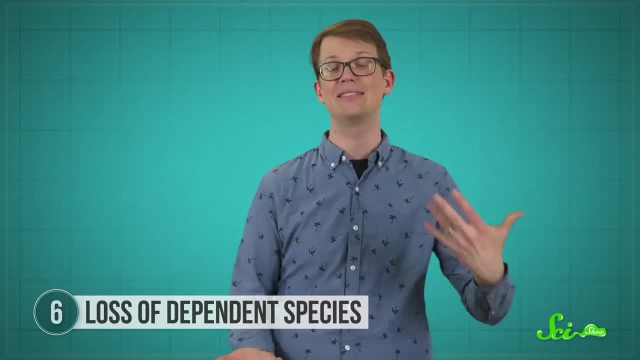 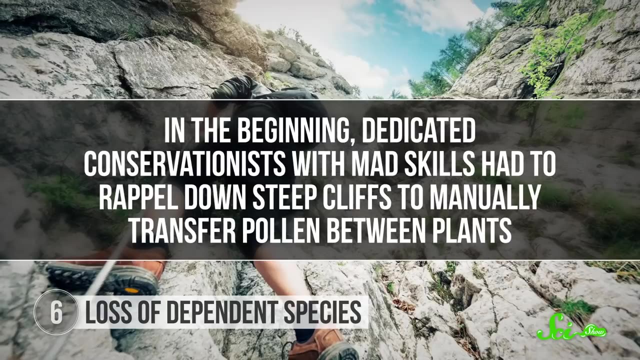 It's a kind of long-tongued moth, But regardless it seems to be gone now. This means that the olula can no longer breed in the wild on its own, so scientists had to step in and help. Of course, these plants do live on cliffs, so this was an extra special kind of rescue. 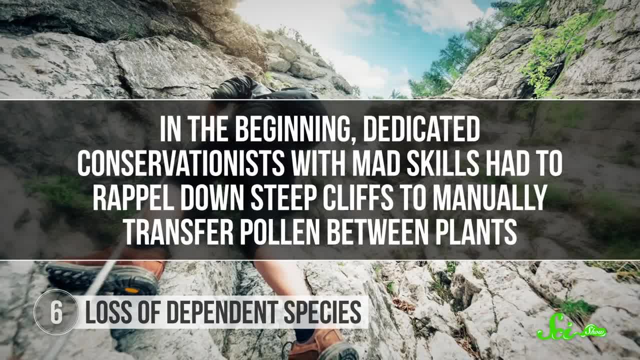 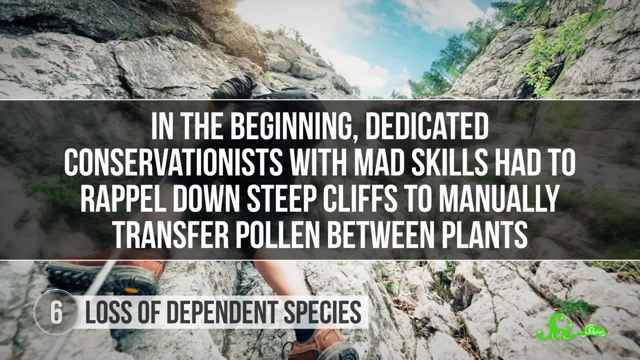 In the beginning, dedicated conservationists with mad skills had to rappel down steep cliffs to manually transfer pollen between plants. just in case you thought biologists weren't hardcore: When these plants produced fruit, they were collected so that the seeds could be grown. 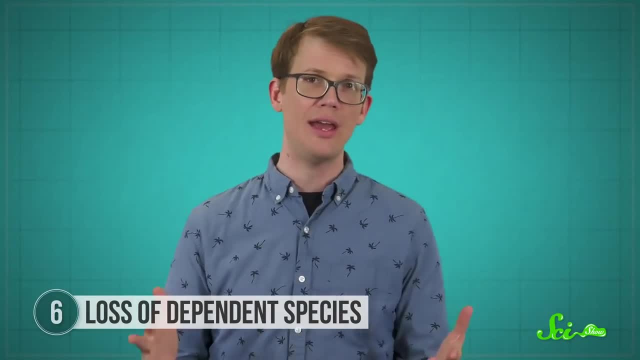 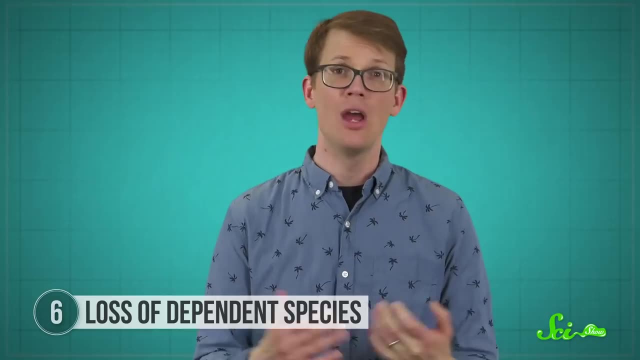 and cared for in greenhouses. The plants haven't been found on Niihau since the 1940s And although there was a population in Kauai, storms wiped it out in the 1980s and 90s. 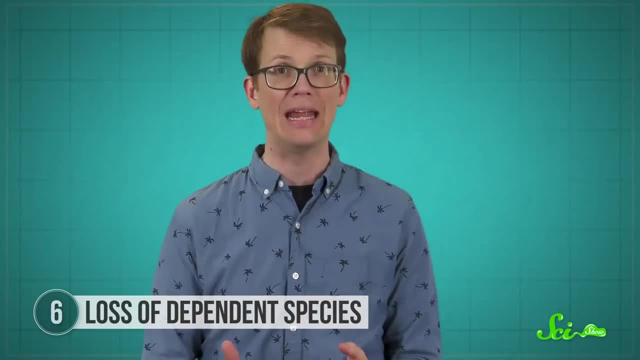 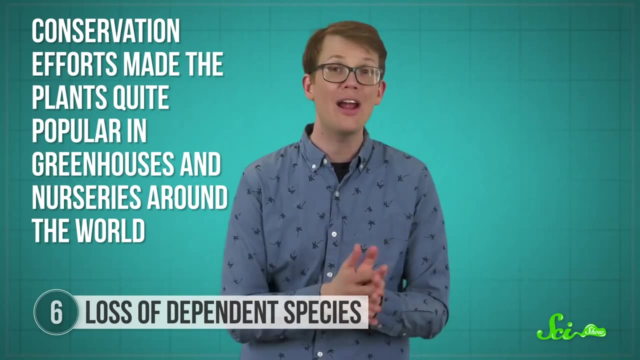 Right now there's only one known wild plant remaining. That being said, conservation efforts made the plants quite popular in greenhouses and nurseries around the world. So they're still out there, And the hope is that eventually they can be planted in the wild again. 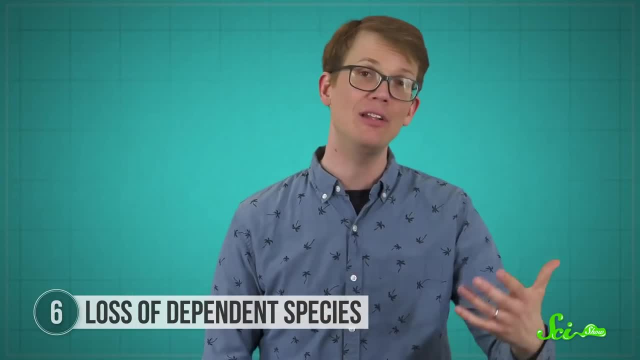 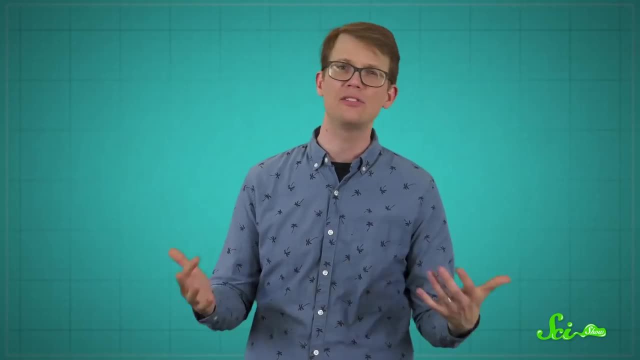 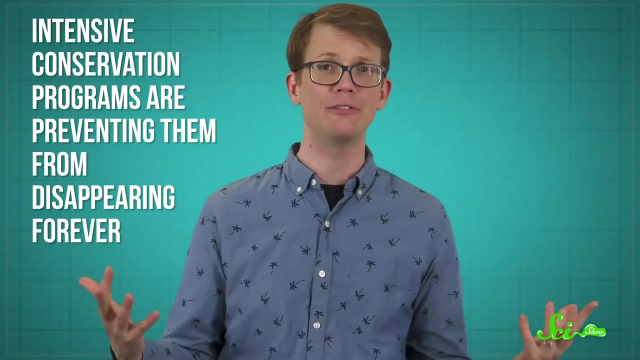 But without a pollinator. this species looks to be heavily conservation-dependent for the foreseeable future. Sadly, in many of these cases the damage has already been done, and some of these species may never thrive without human intervention. But intensive conservation programs are preventing them from disappearing forever, and many researchers 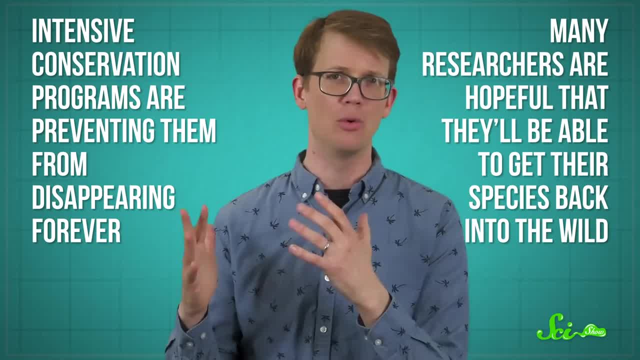 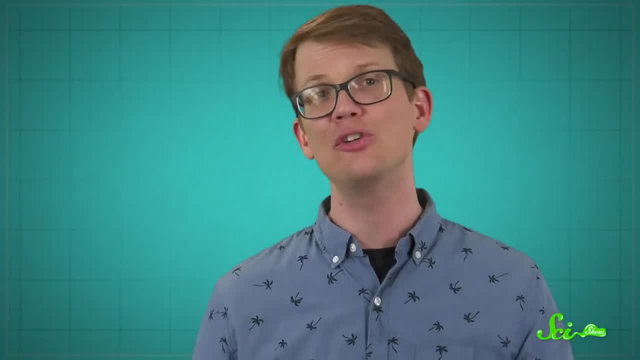 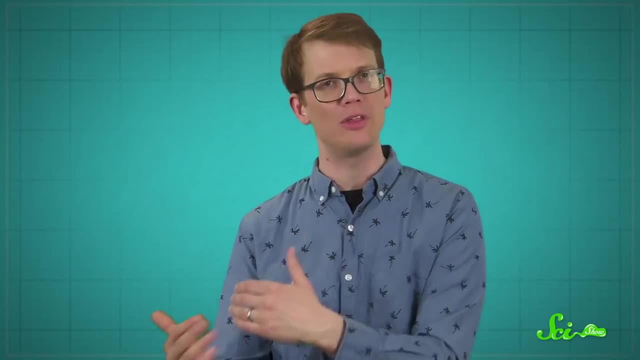 are hopeful that they'll be able to get their species back into the wild. Either way, one thing's for sure: One of the most important factors when it comes to protecting the world's biodiversity is understanding the impact we're having. So, as we keep learning and teaching each other, maybe we'll stop some future problems before. 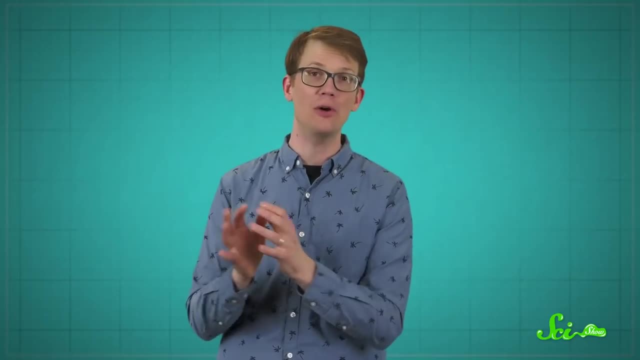 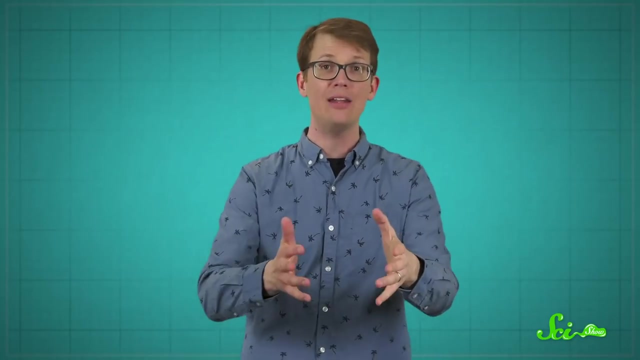 they start. This episode of SciShow is brought to you by our patrons on Patreon, So if you're one of those people, thank you. We couldn't do all this research and production without your support, And your generosity makes a huge difference. 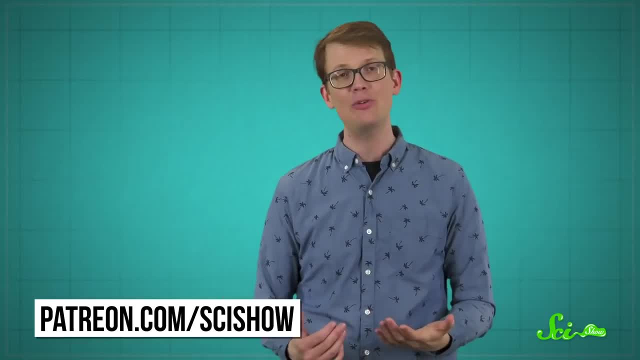 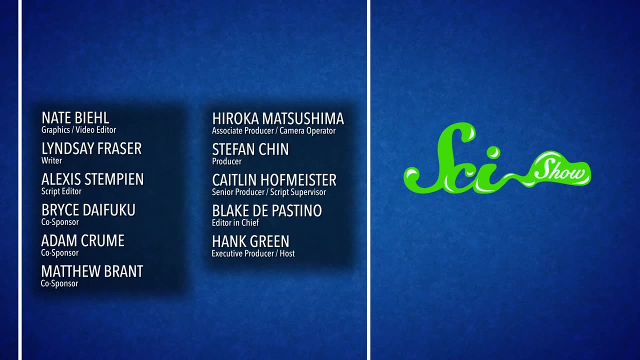 If you want to help us keep making free online content like this, you can go to patreoncom slash scishow. We'll see you next time.